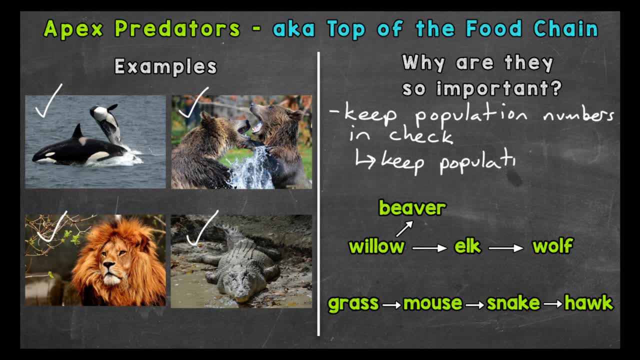 without predators, populations may mainly stay in one area. This again causes everything to be overeaten down to an unsustainable level. Apex: predators keep prey populations on the move. It keeps vegetation numbers at a healthy level and also allows seeds to mature to a well-grown state. I have a great example when it comes to an herbivore population. negatively. 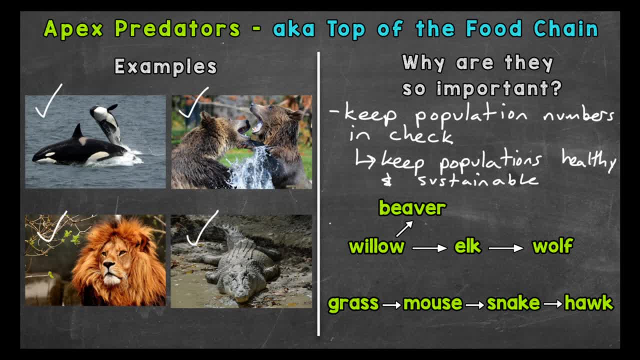 impacting an ecosystem due to overpopulation. To make a long story short, around 1930, all of the wolves were killed off within the Yellowstone ecosystem. Therefore, pressure was taken off the elk population. They were able to stay in one spot more often. The elk decreased the willow population. Beavers use willow to build. 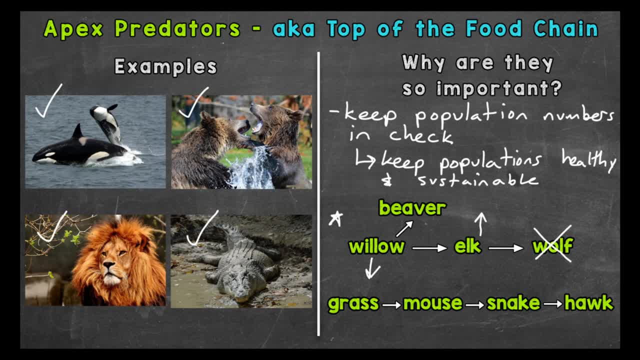 dams and they also eat it. So with the increased elk population there was a decrease in the beaver population. Around 1995, wolves were reintroduced to Yellowstone. This in turn with other factors has helped the beaver population. Apex predators also keep small carnivore populations in check. 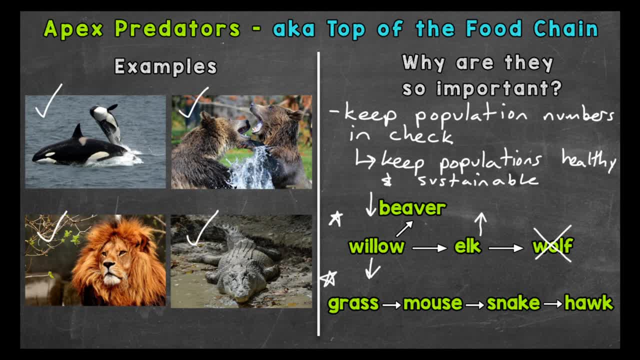 For example. take a look at this basic food chain. So we have grass, a mouse, a snake and a hawk. Let's eliminate the hawk. Without that predator, the snake population would increase. In turn, the mouse population would decrease due to an increase in the snakes. 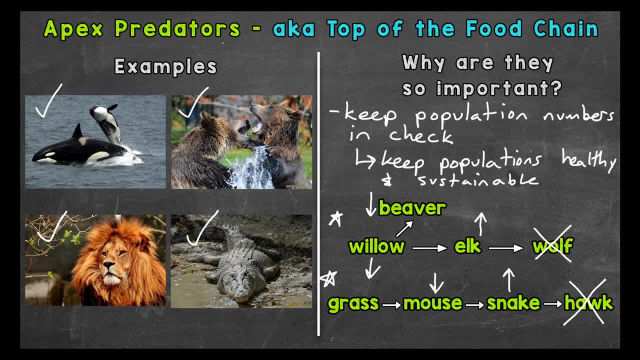 There's nothing to keep the snake population in check. If the snake population got too out of control it could crash the mouse population. That would then crash the snake population. Everything is connected and in balance. The apex predators help keep it that way. 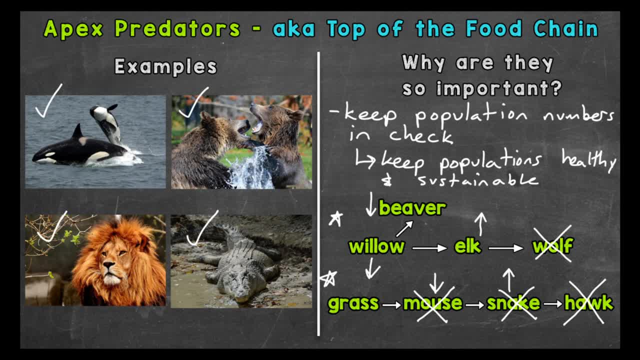 Now, with all this being said, you may be asking yourself: well, what keeps the apex predator populations in check? I will cover that in my next video and I'll drop that link below in the description. For now, know that apex predators are critical to the health and balance. 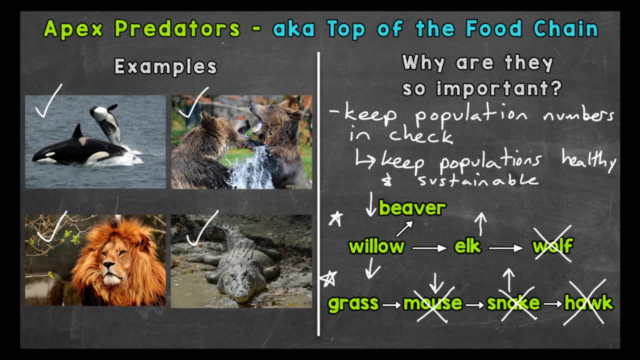 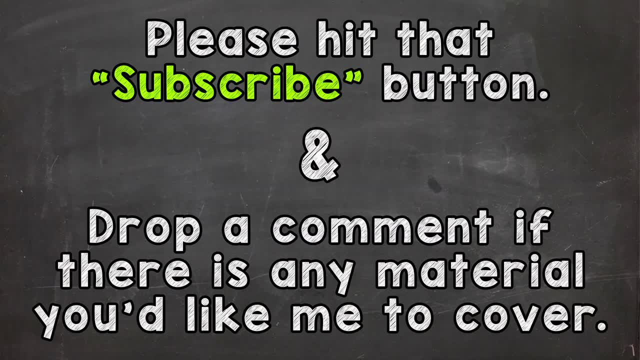 of an ecosystem. So there you have it. There's apex, predators and their importance to ecosystems. I hope that helped. Thanks for watching. Thanks so much for watching. Until next time, peace.